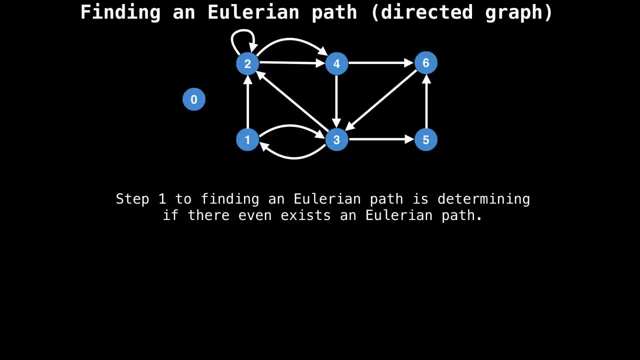 all the edges of your graph And it's good to know that before you actually find your Eulerian path. So recall that for an Eulerian path to exist, at most one vertex has out degree minus in degree equal to one, and at most one vertex has in degree minus out degree. 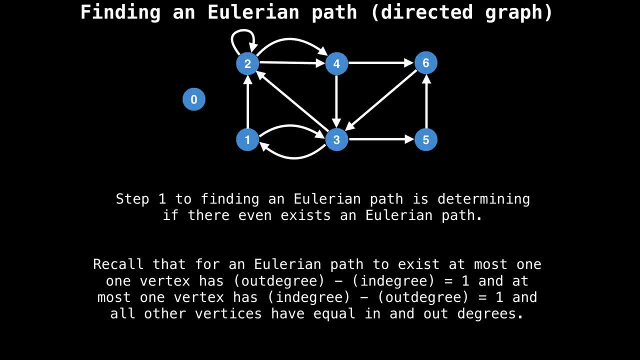 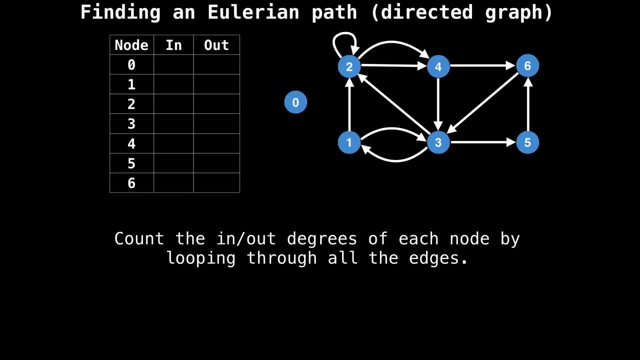 equal to one and all other vertices have equal in and out degrees. we're going to count the in and out degrees of each node by looping through all the edges. we'll be needing two arrays, which I've called Eulerian, In and out, to track the in and out degrees of each node. So for each edge increment, 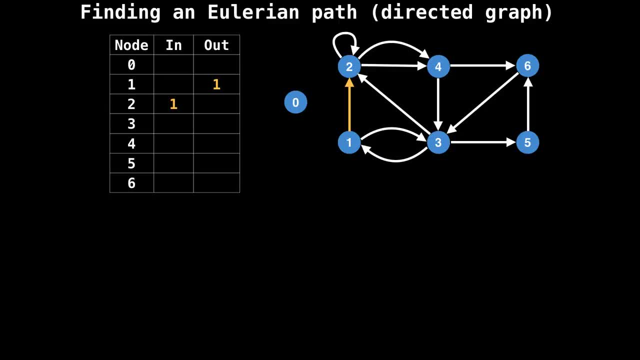 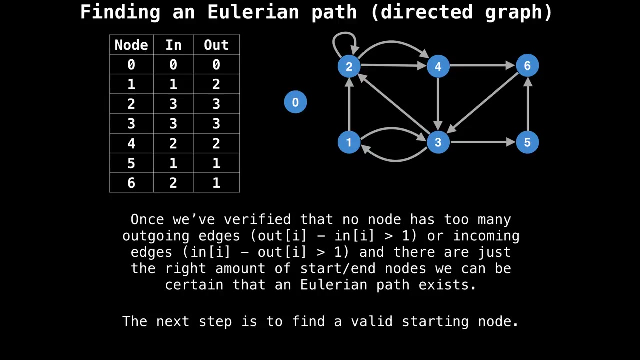 the in degree of a node if a node has an incoming edge, and increment the out degree if it has an outgoing edge, And so on for all the other edges, Once we verified that no node has too many outgoing edges or too many incoming edges and there are just the right amount. 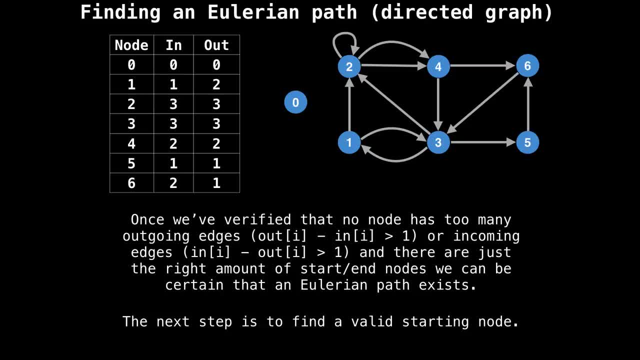 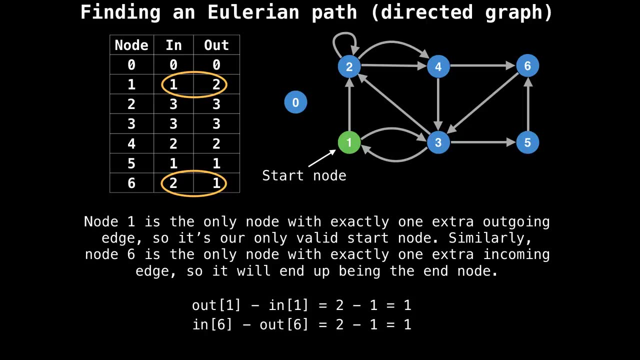 of start and end nodes, we can be certain that our Eulerian path exists. The next step is to find a valid starting node, because we can't start the algorithm at any node we choose necessarily, Node one is the only node with exactly one extra outgoing edge, So it's our 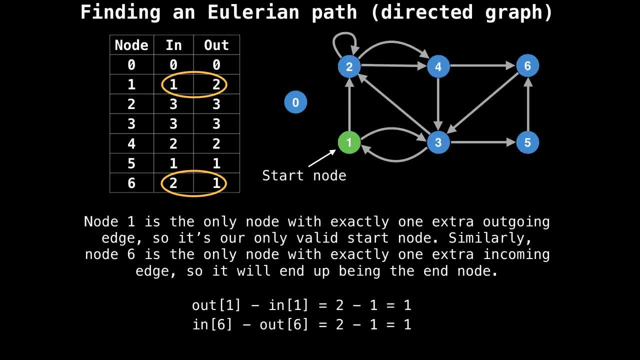 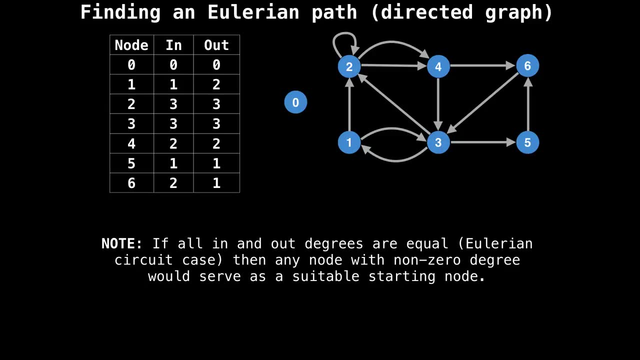 only valid start node. Similarly, node six is the only node with exactly one extra incoming edge, So it will end up being our ended node. Note that if all in and out degrees are equal, then we have an Eulerian circuit And we can choose to start the algorithm at any node which has 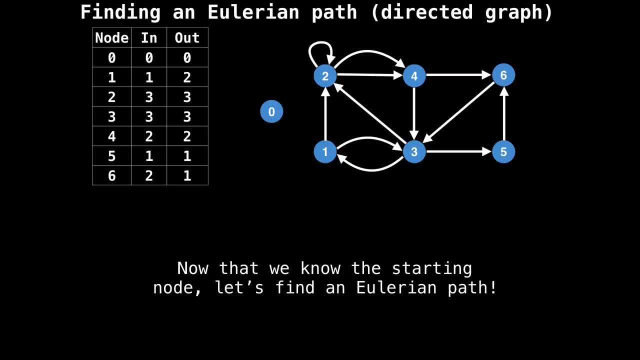 a non zero degree. So we have everything we need to find an Eulerian path. Let's see what happens if we try and do a naive depth for search to traverse as many edges as possible until we get stuck. Let's begin at our starting. 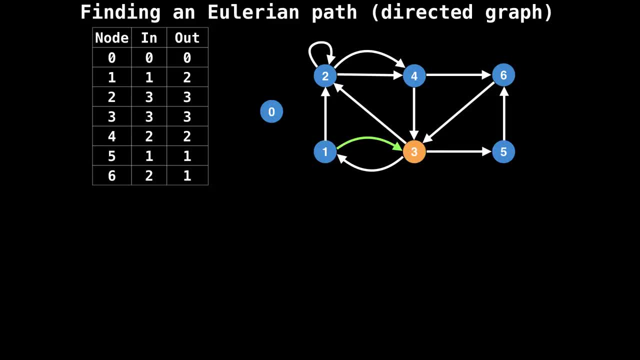 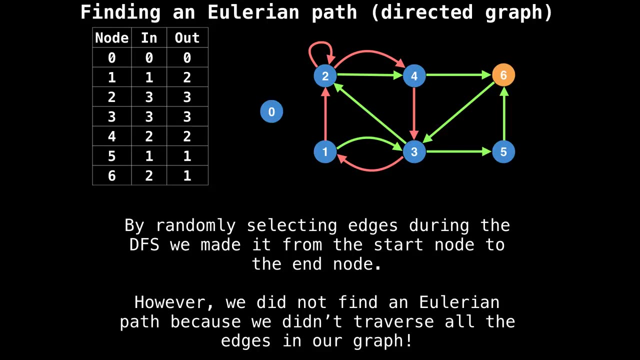 node and execute a random depth for search. Let's take a right, another right, up, down, diagonally, up, diagonally, right and right again. you'll notice that, even though we started at the correct starting node and that we knew an Eulerian path existed and furthermore, 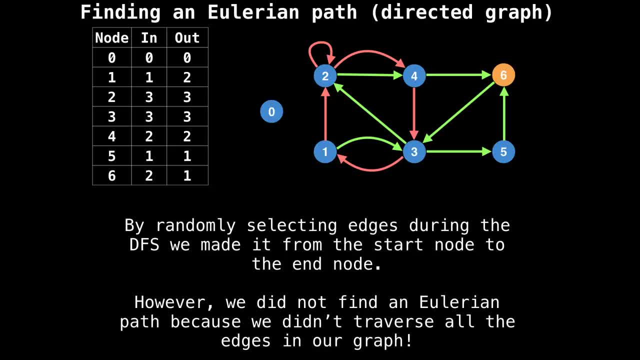 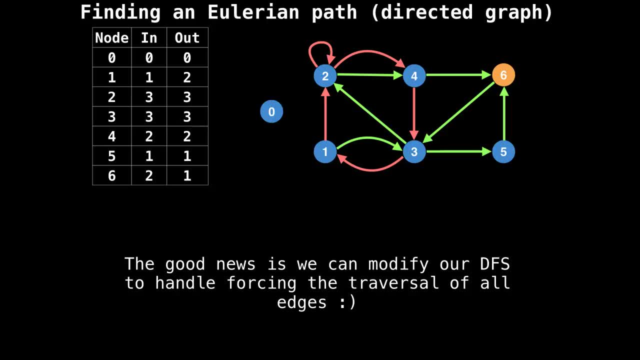 that we did end up at the correct end node, that we still did not find a valid Eulerian path, since we didn't traverse all the edges. So what's going on? Well, what's happening is that we're doing our depth for search wrong. we need to modify the depth for search algorithm to force the depth for 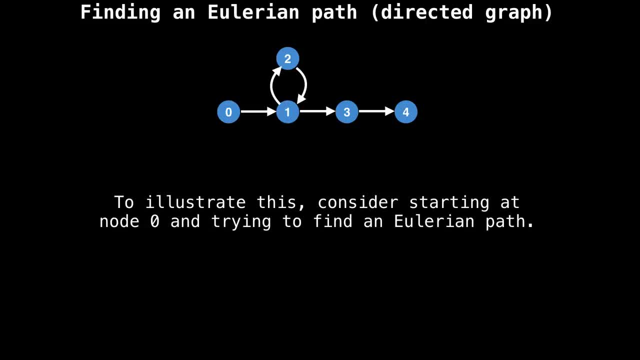 search to visit all the edges of our graph. To illustrate this, consider this simpler, smaller graph. Suppose we start our depth for search at node zero and try to find an Eulerian path. Suppose we take the edge to the right. then suppose: 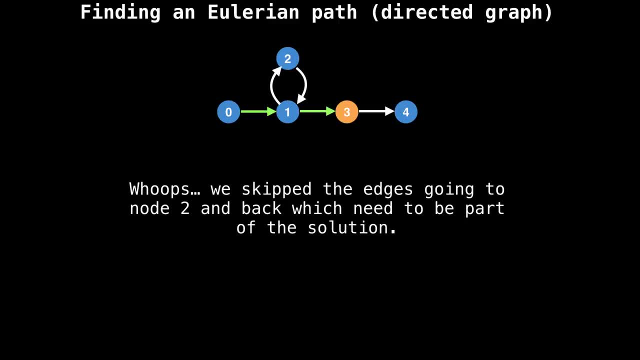 the depth for search takes us right again. this causes us to accidentally skip the edges going to node two and back, which we know will need to be part of the Eulerian path solution. For now, let's not worry about it and keep executing our depth for search. So 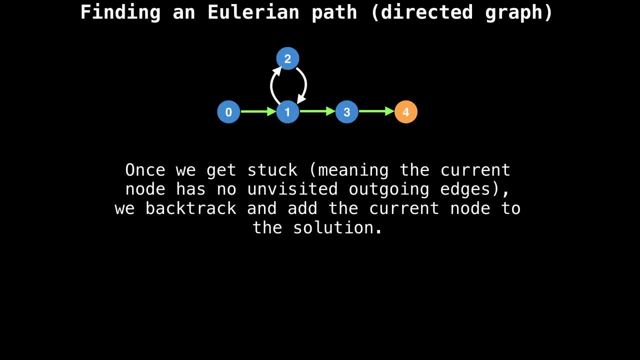 once we get stuck- meaning the current node has no unvisited outgoing edges- we back to track and add the current node to the solution. So for gets added to the solution and we return to the node we were just at. we are stuck again because node three has no outgoing 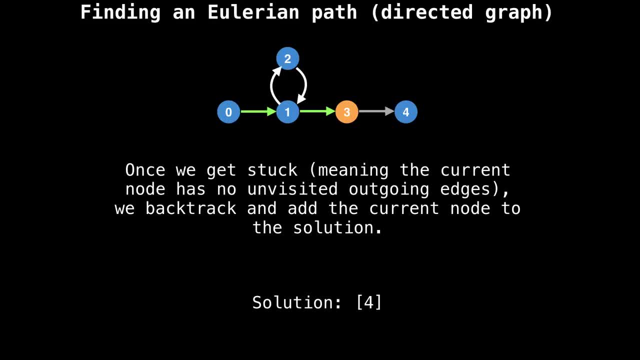 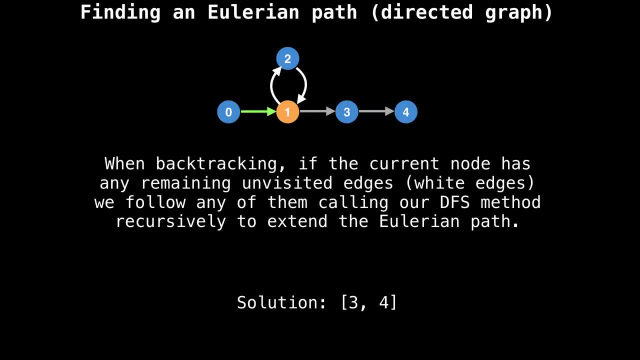 edges that are unvisited. So we add three to the front of the solution and backtrack. When backtracking, if the current node has any remaining unvisited edges, that is, white edges, we follow any of them, calling our depth for search method recursively to extend the 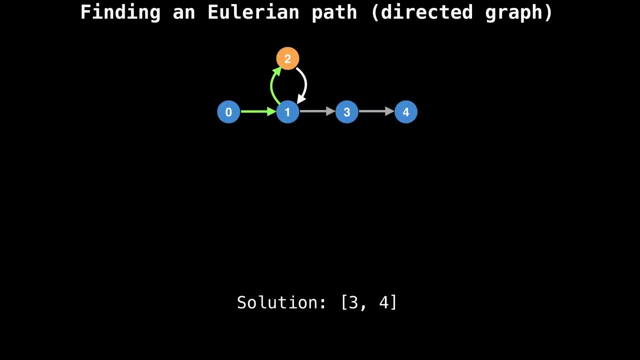 Eulerian path. So we follow the edge up to node two, and then there's still another edge going downwards, So we take that one too. Now we're stuck again because there aren't any unvisited edges anymore. What we do is we backtrack and add the current node to the front of the solution Effectively. 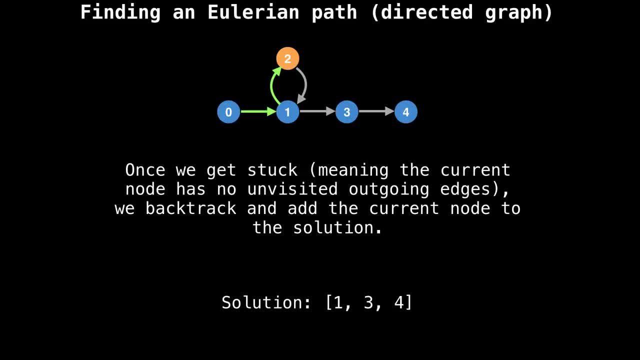 we do this until we return to the start node and the recursion unwinds. So, in summary, how we force the depth first search to take all the edges is to keep taking unvisited edges on the recursive callback until no unvisited edges remain Coming back. 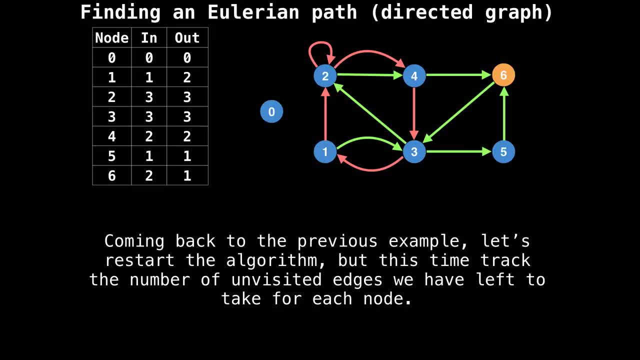 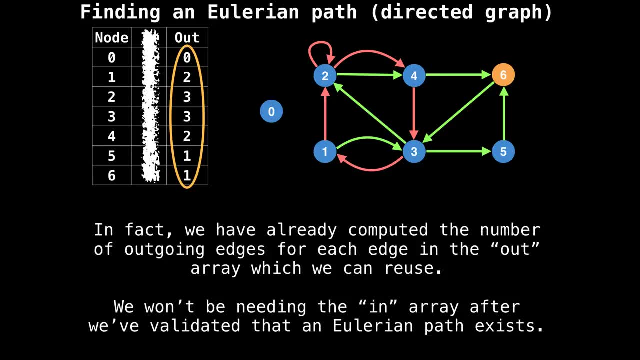 to the previous example. let's restart the algorithm, But this time let's track the number of unvisited edges we still have left to take at each node. In fact, we have already computed the number of outgoing edges for each node in the out array which we can reuse. 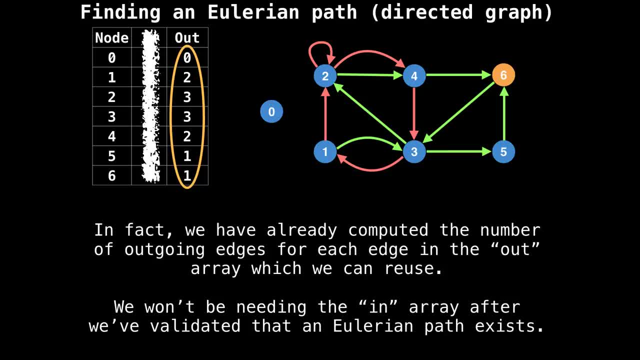 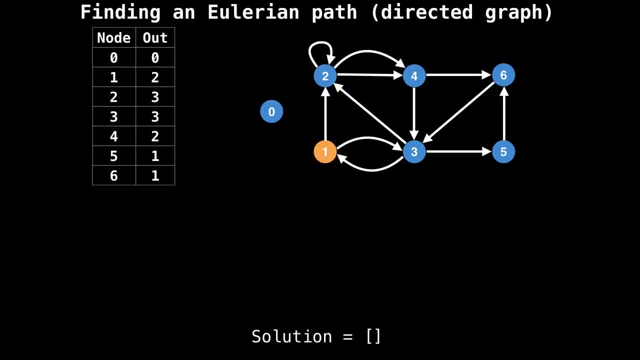 we won't be needing the inner array anymore. Once we validated that an Eulerian path, we're going to see that the path exists, So we can ignore it. Let's begin at the starting node once again Now. one thing we're going to do slightly differently is that every time, 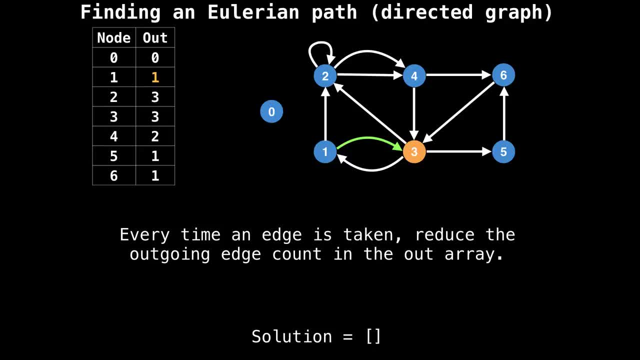 an edge is taken, we'll reduce the outgoing edge count for that node. Doing this will enable us to know when a certain node has no more unvisited edges. So let's just follow the same path we had last time until we get stuck. 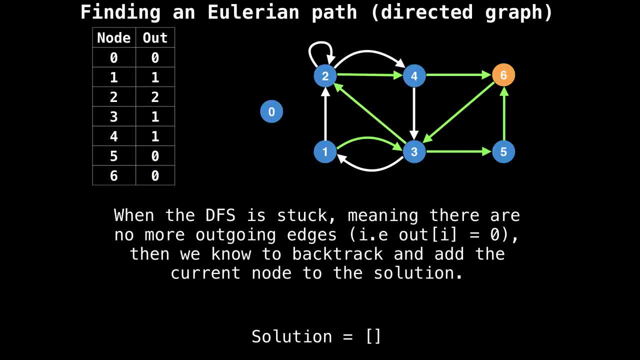 Okay, so now we are where we were last time, but we're not going to terminate the algorithm just yet. Instead, we're going to backtrack because we're stuck and there are no more outgoing edges to take from node six. One way to know this without looking at the graph: 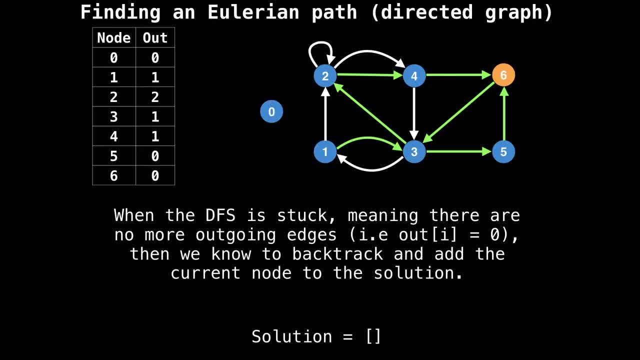 is to check whether the out array at index six has a value of zero, and it does. So let's backtrack and add six to the front of our solution. Now we are at node four, and node four has remaining unvisited edges. Those are the white. 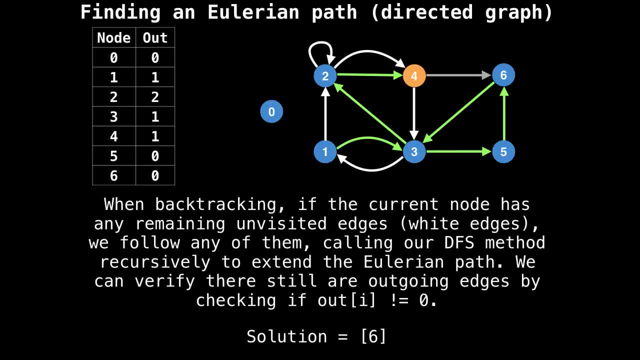 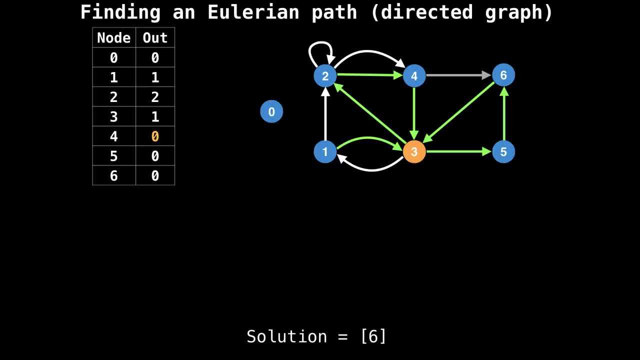 edges which we still need to take. So we call our depth first search method recursively and follow all the unvisited edges. for node four, similar situation at node three and node one and node two. For node two we're going to take the edge going to the right. 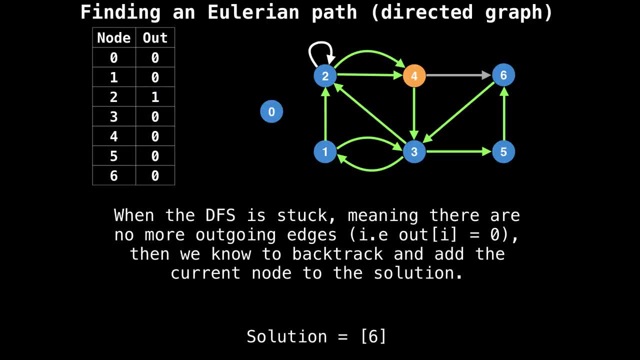 which brings us back to node four, But this time there are no more outgoing edges. So we're going to take the edge going to the right, which brings us back to node four, But this time there are no more outgoing edges to take from node six. One way to know this: 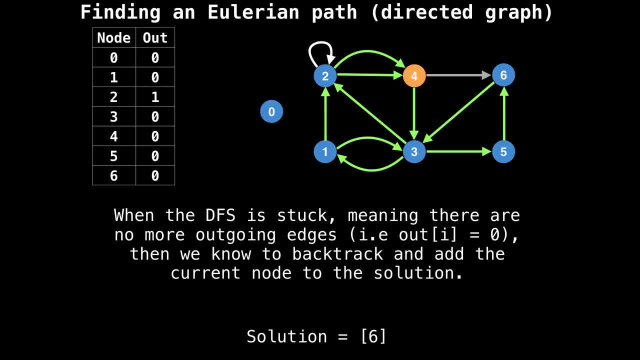 without looking at the graph, is to check whether the out array at index six has a value of zero, which brings us back to node two. And because it was negative, we are going to stack and see that we now have no more unvisited edges at node four. So what do we do? we backtrack. 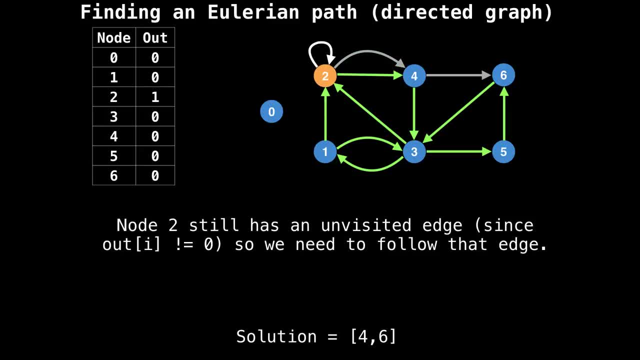 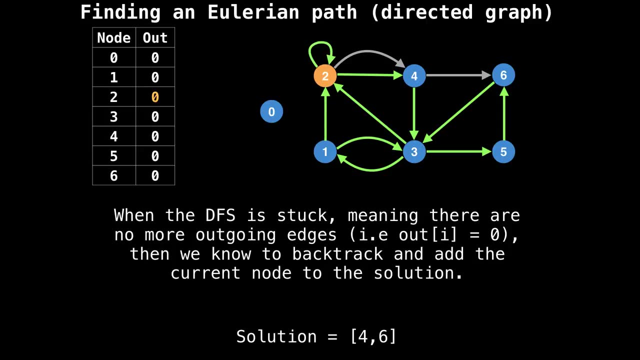 and add four to the front of our solution. Now we're at node two, and node two still hasn't unvisited edge, since the out array at index two is not equal to zero. So what we do is we follow that unvisited edge, which brings us back to node two, and node two now has. 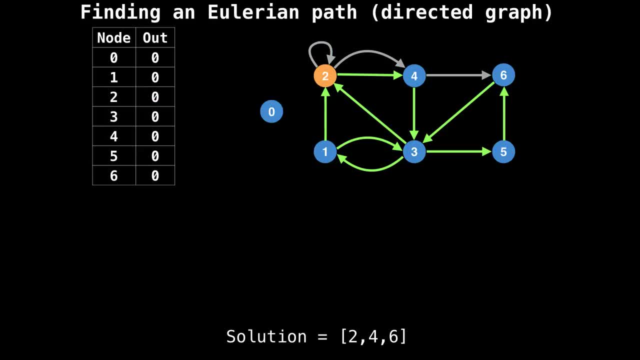 no more unvisited edges. So we backtrack that to the solution and we're back at node two and backtrack until we make the right choice. But not only that. you're going to set the and we backtrack. Now we're at node one and backtrack from node one. Now we're at node. 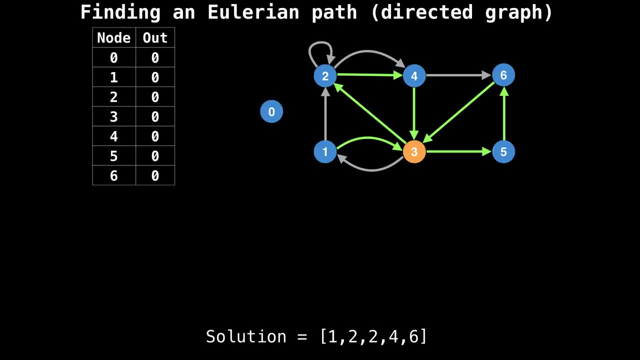 three and so on. since all the edges have been visited, And at this point we're just going to unwind the stack and add the current node to the front of the solution, I'll let the animation play. And that's how you find an oil arian path on a graph, In terms of 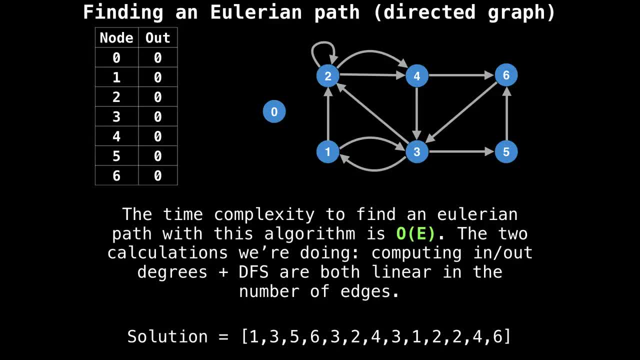 the time complexity required to find an oil arian path. we know that it has to be big O of E. The reason is that the calculations we're doing to compute the oil arian path are all linear in the number of edges. Think about computing the in and out degrees, or 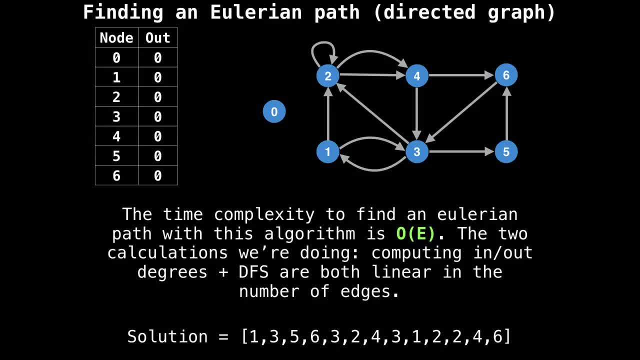 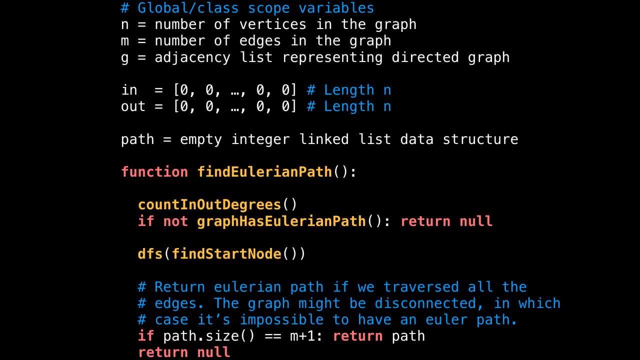 the depth of research. both of those only take big O of E time. So the whole thing is linear in the number of edges. And now let's have a look at some pseudocode to find an oil arian path. Let's have a look at some of the variables we're going to need, The first three here. 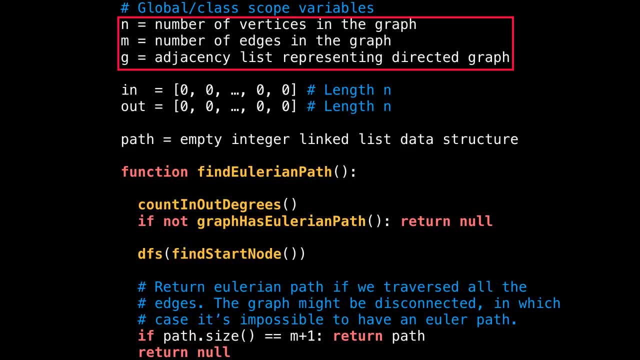 are inputs to the algorithm, which are: n- the number of nodes in the graph, m- the number of edges in the graph And, lastly, G, the graph itself stored as an adjacency list. Then there's the in and out arrays I talked about earlier to track the in and out degrees. 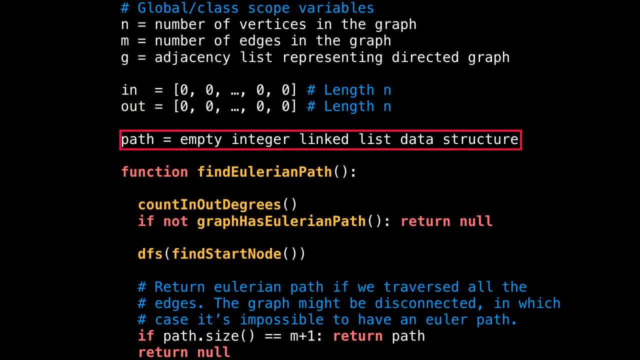 of every node. Lastly, there's a variable called path, which is a linked list which is going to store the oil arian path solution. You can also use an array or some other data structure to store the solution, But I find that a linked list simplifies the code to actually find an oil arian path on. 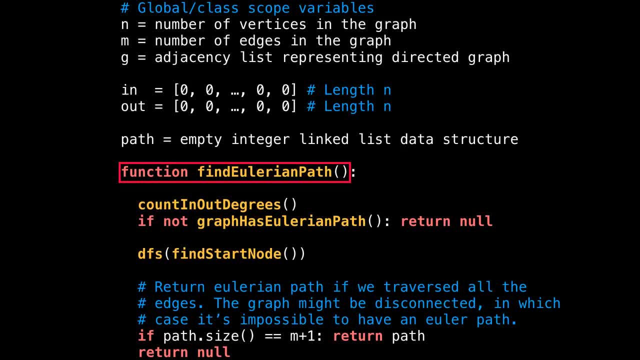 our graph G we're going to call the find oil arian path method. The first thing we want to do is verify that an oil arian path exists. To do that, we first need to count the in and out degree of each node And once 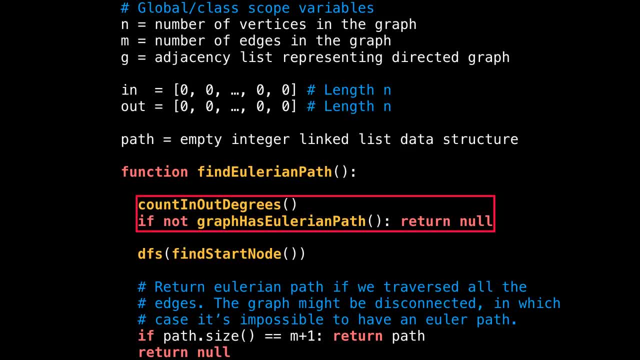 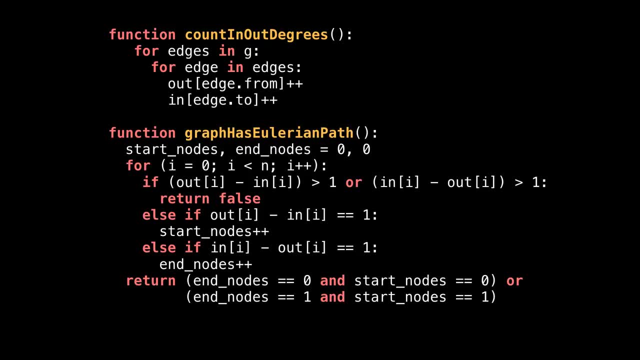 we know that we can verify that the graph is a good candidate for an oil arian path. So here we are, looking at the methods which count the in and out degrees of each node and verifies that oil arian path can exist. The count in and out degrees method is very 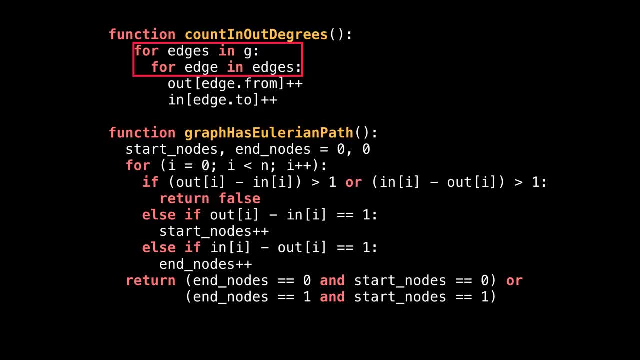 simple. Simply loop over all the edges in the graph and increment the in and out degree array arrays for incoming and outgoing edges. The graph has oil arian path method. checks all the preconditions for an oil arian path. we're going to keep track of the number of start. 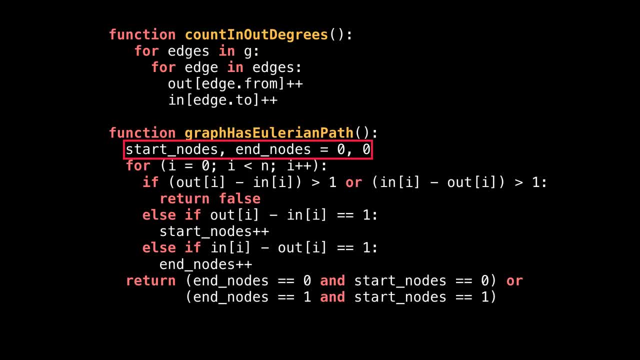 nodes and end nodes that we encounter. a start node is a node with one extra outgoing edge and an end node is a node with one extra incoming edge. If, at any point, we encounter a node which either has more than one extra outgoing edge or more than one extra incoming edge, we know that. 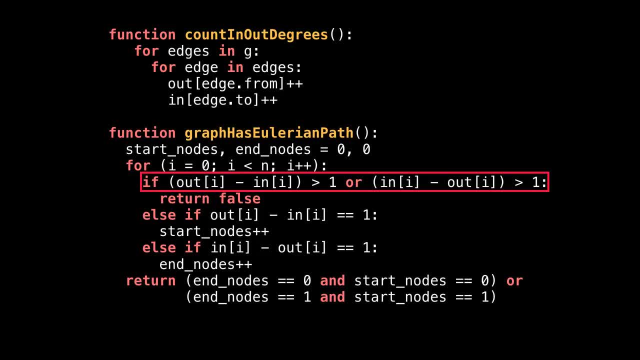 this graph is not oil arian and we can return false immediately Because of symmetry. I believe you only need one of these checks. But to be explicit, I put both conditions there. Next up, I check if the current node is a start node or an end node. you cannot. 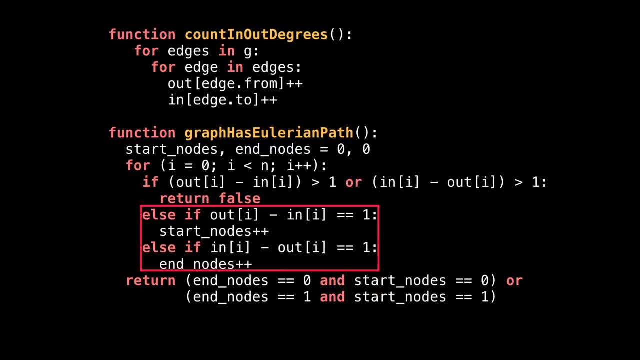 be a start node and an end node, which is why this is a start node. This is an else if clause. the last thing to do is check if we have a valid number of start nodes and end nodes for our path. Either there are no designated start and end nodes. 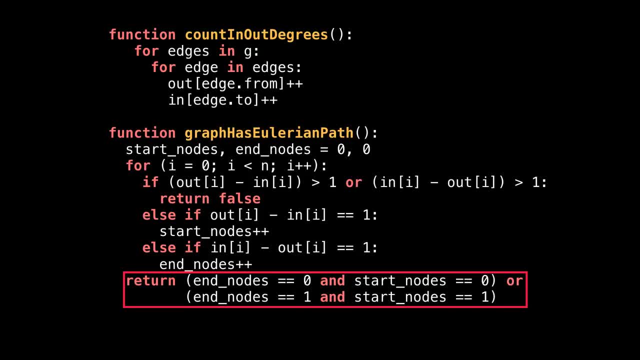 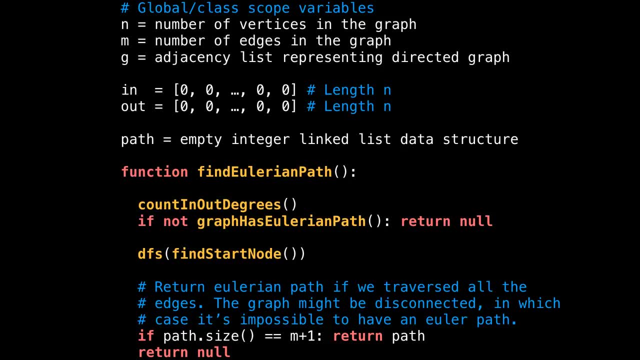 that is the oil arian circuit case, which is also an oil arian path, or there are exactly one start node and one end nodes. Coming back to the main method, the next step is to find that starting node and perform a depth first search to actually find the oil arian path. 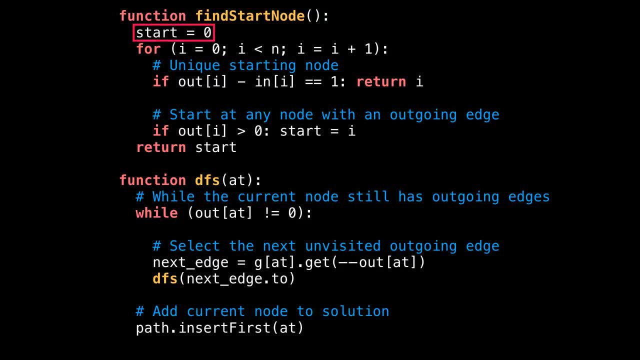 Let's begin with finding the starting node. we're going to start by assuming that the start node is node zero, Although this will likely change in the future, Since we know that at this point, our graph is an oil arian graph. This means that if we encounter a node, 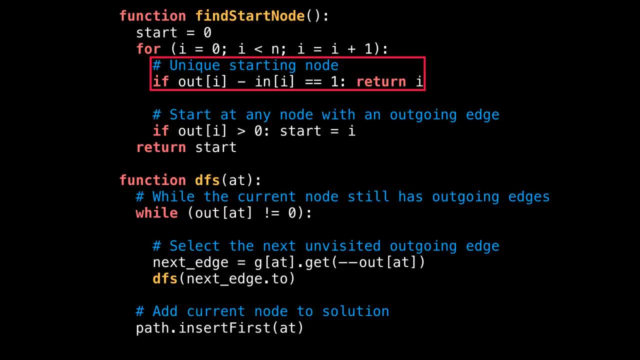 with one extra outgoing edge, that this node must be the unique starting node and we can return that nodes index immediately. Otherwise, we just want to ensure that we begin on a node with an outgoing edge. our default node, node zero, might not have an. 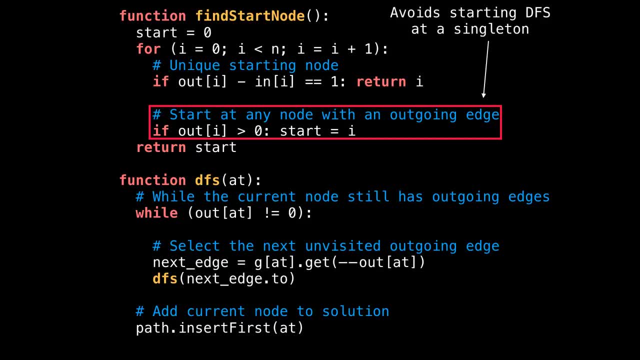 outgoing edge. In fact, this check prevents us from starting the depth first search on a singleton node, then return the start node after the loop. the depth first search method is where things start to get interesting. This depth first search method takes one argument. 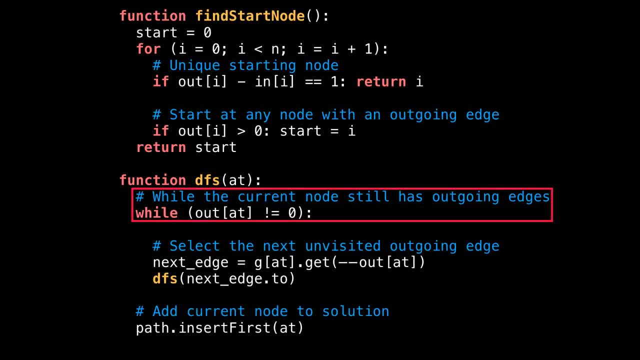 And that is the current node. we're at the while loop in the depth. first search loops, while the current node still has outgoing, unvisited edges. It does this by looking in the outer array at the current node and checking if there are still outgoing edges. The next: 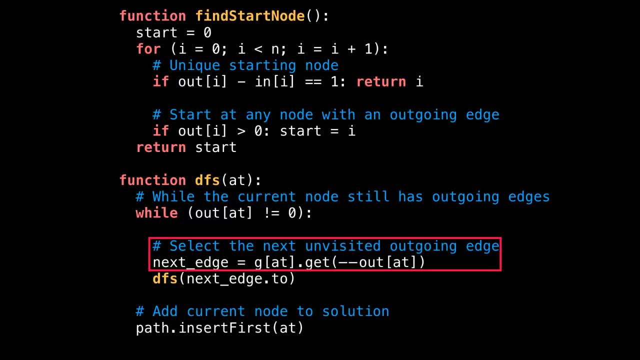 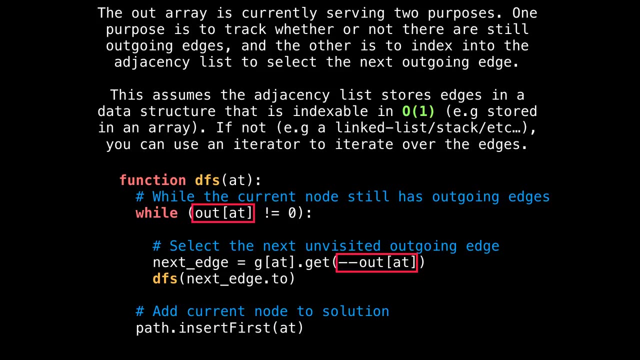 line selects the next unvisited outgoing edge from the current node from our adjacency list. It also decrements the number of outgoing unvisited edges from the current node. So if you haven't caught on already, the out array is currently serving two purposes: The 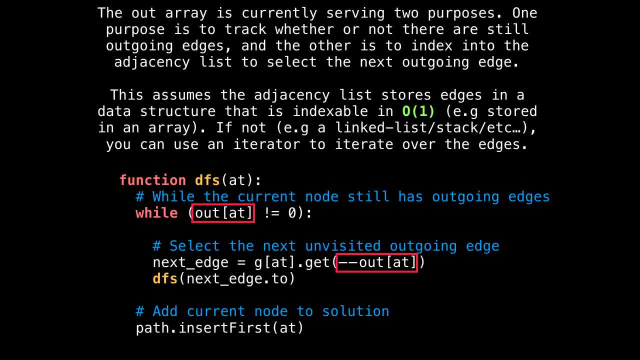 one purpose is to track whether or not there are still outgoing edges And the other is to index into the adjacency list to select the next outgoing edge. This assumes the adjacency list stores edges in a data structure that is indexable in constant time, just like in. 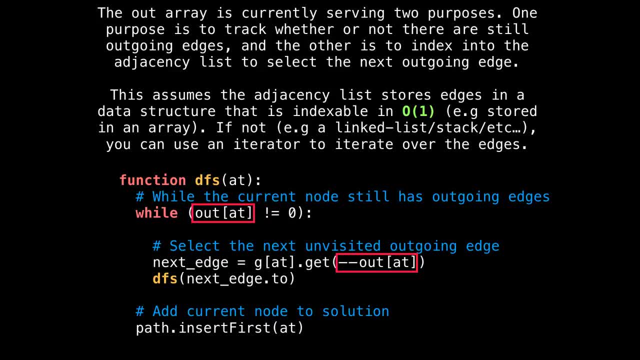 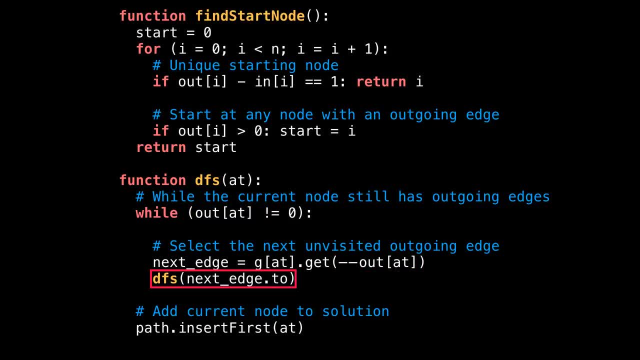 array. If not, say, you're using an adjacency list composed of linked lists, then you can use an iterator to iterate over all the edges. Once we've selected the next unvisited edge, we can then start writing out the string type ofados That is, we'll need to write any top. 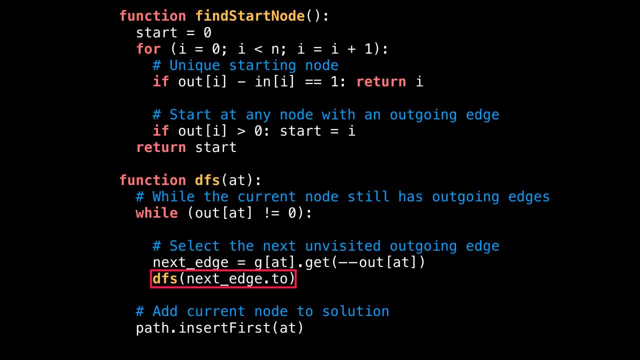 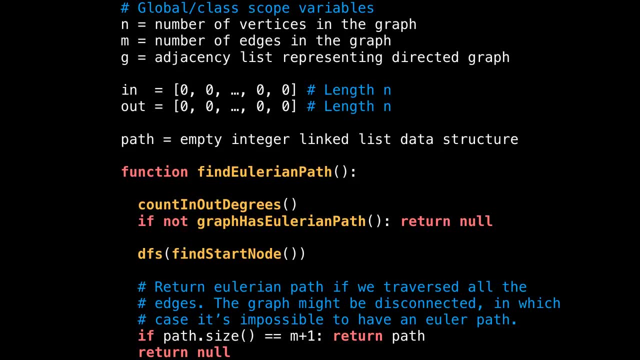 visited edge. we visit that edge by calling the depth first search method recursively. Once we exit the loop, append the current node to the front of the solution. Returning back to the main method, the last thing we need to do is check that we have actually. 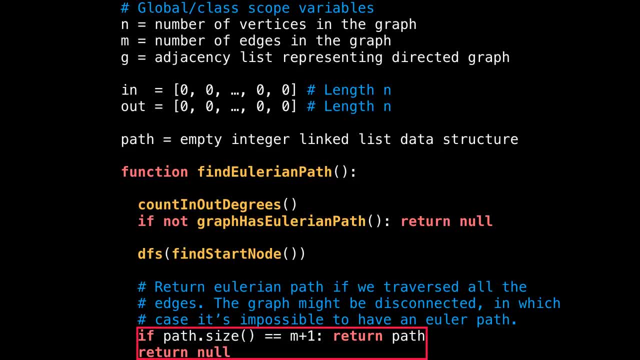 found the correct number of edges for an Eulerian path. it might be the case that our graph is disconnected and we found an Eulerian path on one of the many connected components of our graph, in which case it's impossible to actually have an Eulerian path. So we return. 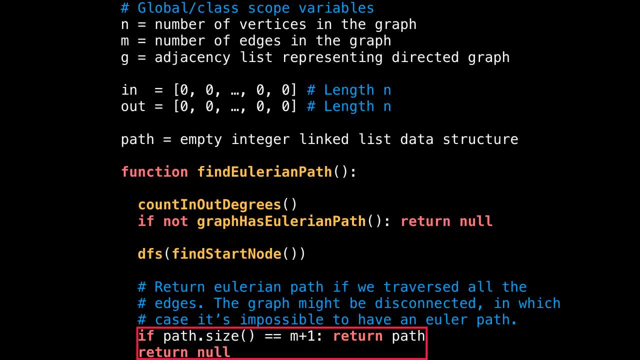 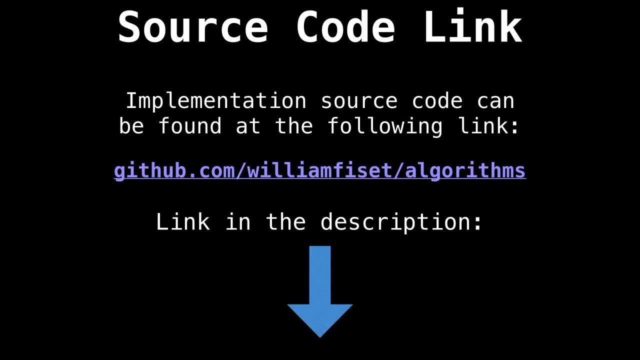 null in that case. Otherwise, we simply return our path. All right, everybody. thank you for watching. As always, you can find source code on GitHub at githubcom. slash- William Fiza slash algorithms. there should be a link in the description. Please give us a like. 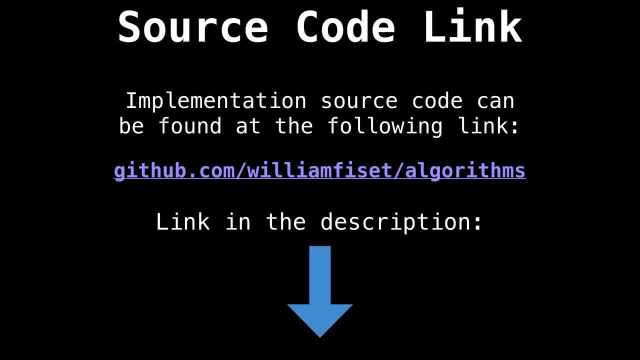 and subscribe And, as always, thanks for watching And we'll see you in the next video. Bye, Give this video a thumbs up if you learned something, and subscribe for more mathematics and computer science videos.